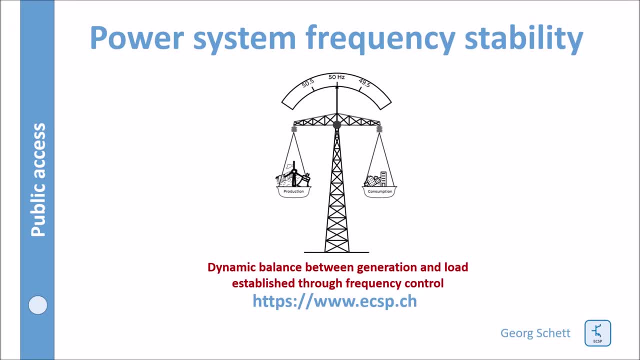 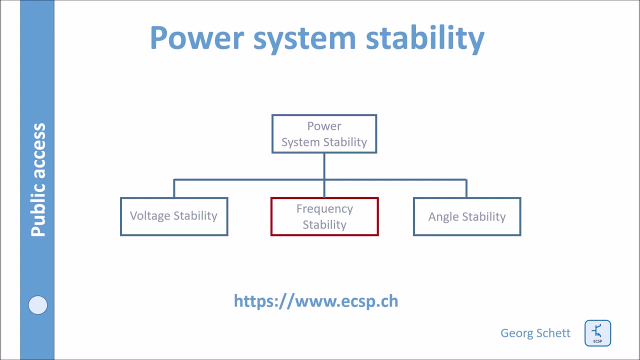 In the electric system, the balance between power generation and load must be guaranteed all the time. If not met, serious consequences such as blackouts may occur. The balance between generation and load is met by controlling the frequency of the system. The frequency stability is one of three criteria which have to be met all the time in order to keep the system stable. 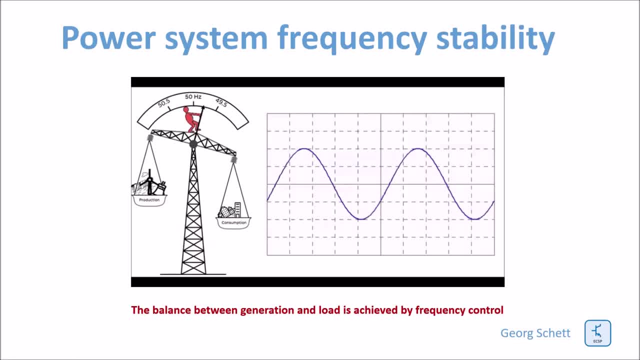 If the load exceeds the power supplied by the generation, the system frequency will be slowed down, and vice versa. It is like a car where the force of the brakes exceeds the torque of the motor. The equilibrium is met by a sophisticated and decentralized control system. 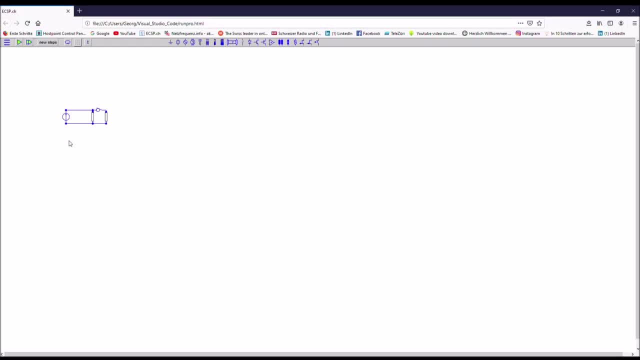 On my homepage there is a very simple model attached. You can run it so you can train your skills as an operator. The model consists of a power generation- It is just one phase- Then a variable load consisting of one fixed load and a second load which is connected and disconnected by means of a random switch. 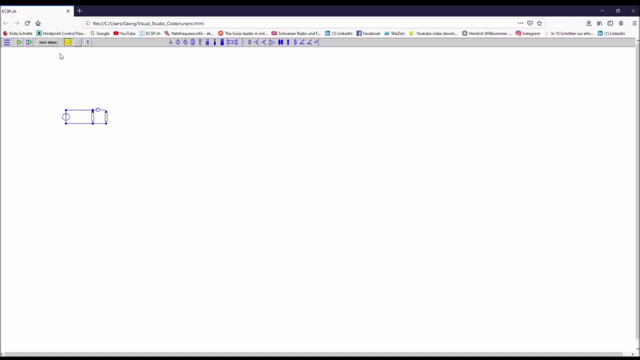 In order to operate it, you first put the infinite load to yellow, Then you push the green arrow button, You relocate the curves, Then you adjust the position of the frequency meter, Then you start the process, Then you quickly push the power up. 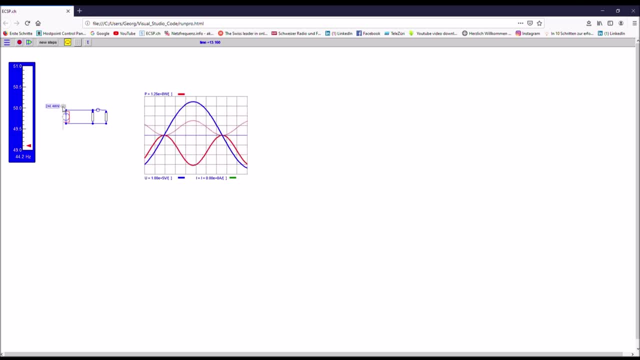 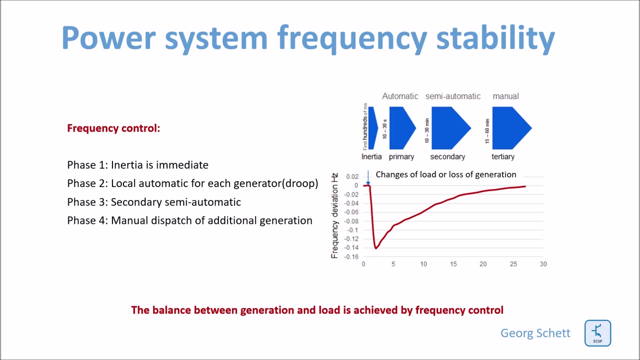 The frequency of the system comes back to 50 Hz, where it should be. Then you push up and down this arrow here. Then you can compensate for the changes in the load which is, with this random switch, Play the operator's game. The frequency control is performed as follows. 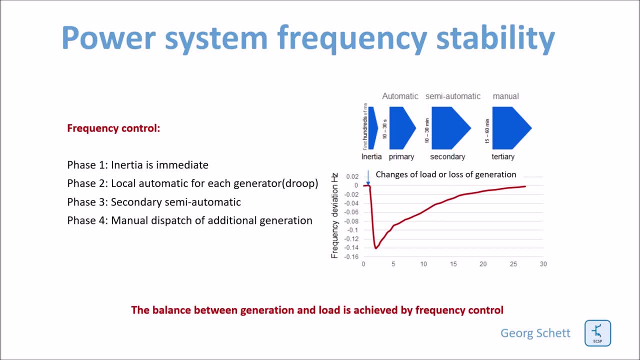 After a change of the load or a loss of generation, there are three consecutive phases. The first phase- phase 1, is immediate And in this phase the demand is met by using the stored energy in the rotating mass of the generation involved. 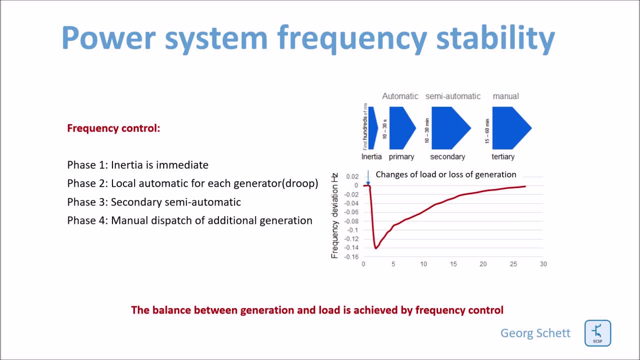 Or if the generation exceeds the load, the energy produced is stored in the rotating masses. That means the rotation speed is accelerating. The frequency goes up. In a second phase there is a very local generation control. It's the so-called droop which is opening or closing the valves, for example, of steam engines or of hydro power plants. 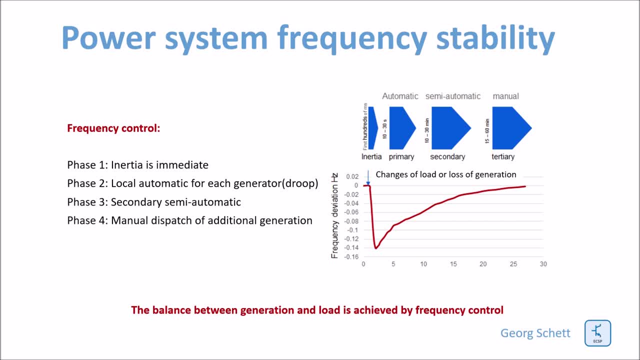 In the third phase there is a regional control system which controls the droop settings of the generators And with this regional control the region can fully meet the frequency, the momentum frequency. In the fourth phase there is maybe additional generation which has to be set up and connected or disconnected to the grid. 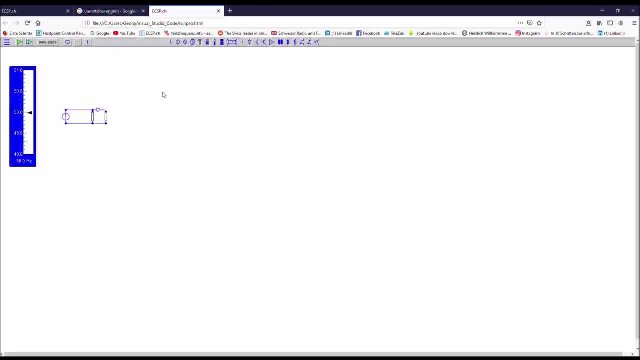 In the previous exercise we have seen that it was quite tough to control the frequency manually And therefore we want to have some support now by this so-called droop of the generator. You see that there is a push button here. You can click it and then you get some support to control the speed of the generator. 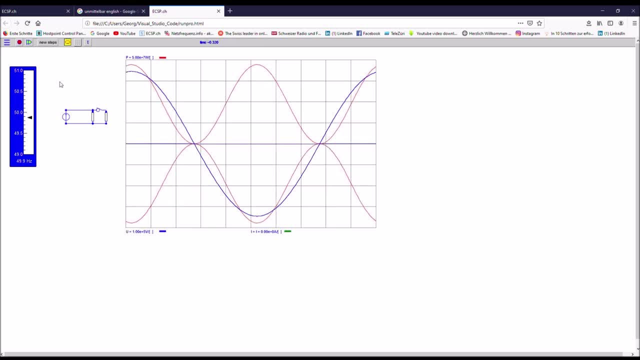 Again. you go here and you see now that the frequency remains relatively close to the nominal, even with the change in the load, And so the only thing you have to do now is to adjust the frequency manually. This would normally be done by the automatic grid controller. 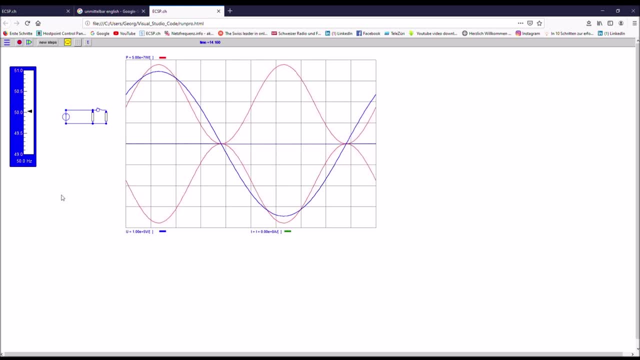 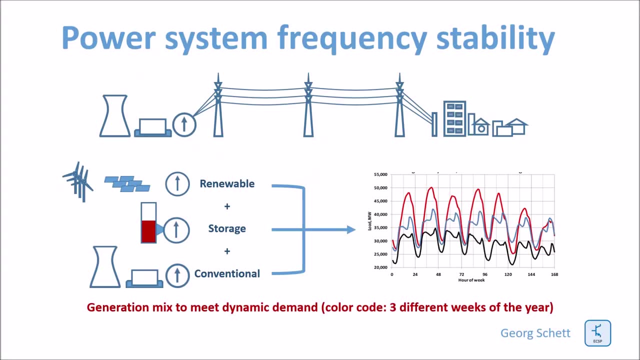 And you see that it's now much, much easier. So you switch on the droop and then you have much less stress. Today the power system is starting to be quite complex, So you see typical demand patterns during three different weeks of operation. 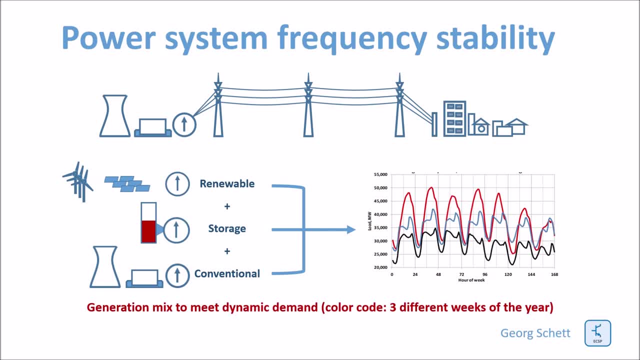 For example, you see the daily pattern of a year. You see the seven days per week and you see how the daily pattern works all across the week. It's very similar during all the days in the year. However, there is some changes in the maximum and minimum. 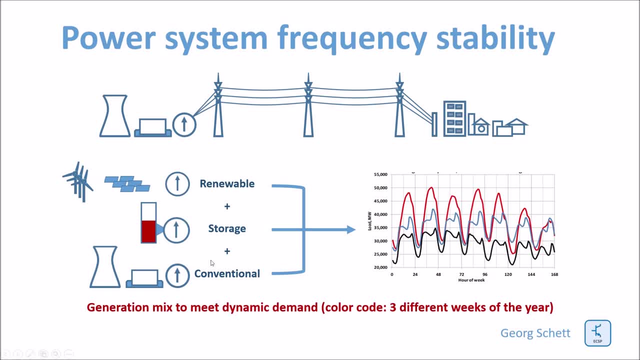 What is difficult today, more and more, is that the power generation is less and less controllable, Because there is more and more renewable power, which feeds power into the grid, And the renewable power, as we all know, is not that well controllable. 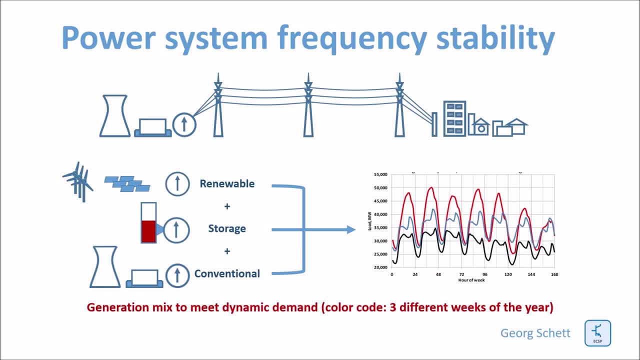 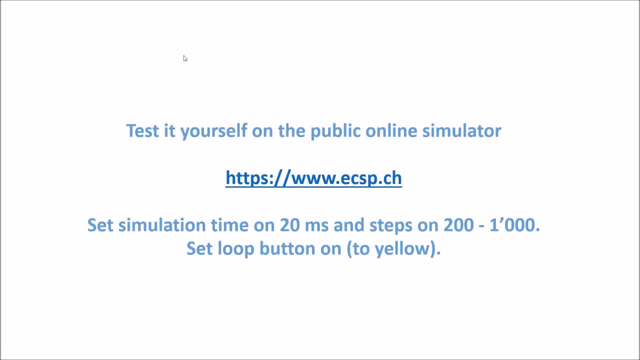 The wind blows or it doesn't blow when you need the power, And therefore the storage is more and more important and the grid connections is more and more important. If you go to my homepage, you can play around with the generation and gradually learn to be a very good grid operator. 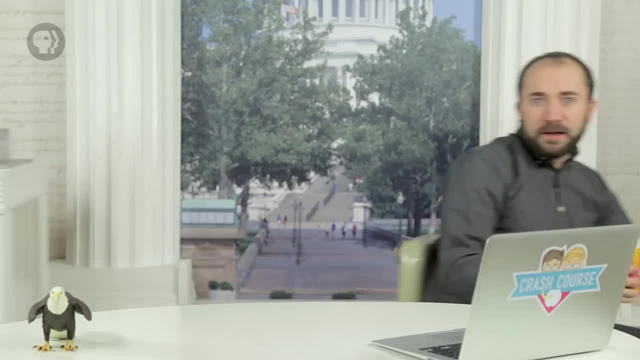 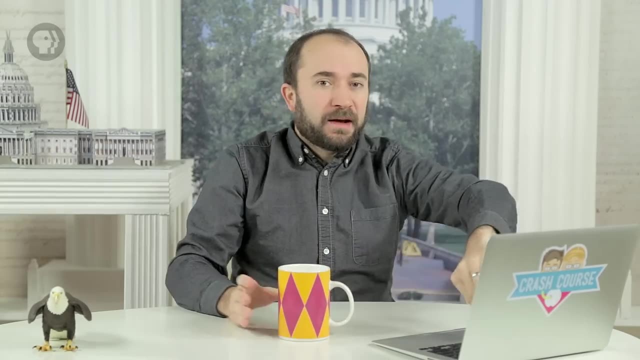 Hello, I'm Craig and this is Crash Course, Government and Politics, and today we're finally going to talk about a topic I know that you've all been waiting for: monetary and fiscal policy. Hooray, You haven't been waiting for monetary and fiscal policy, Are you sure? 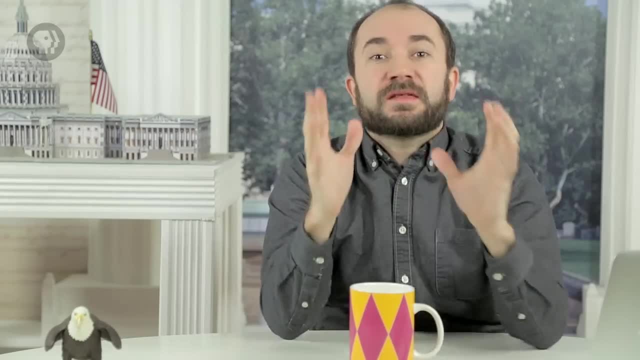 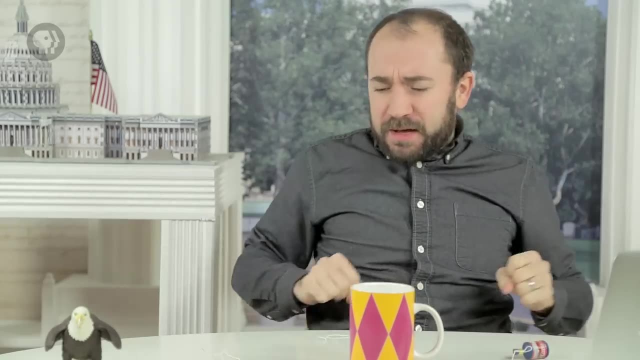 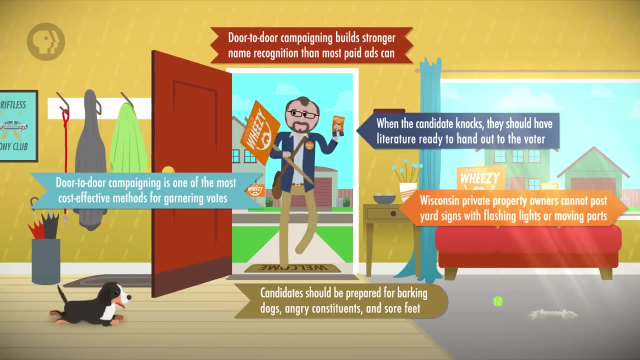 I've been talking it up for weeks, you know. Well, let me see if I can't convince you to be as excited as I am. Monetary policy, Woo, Fiscal policy. yeah, I wanna get fiscal, fiscal. Come on and get fiscal. Okay, let's start the show. 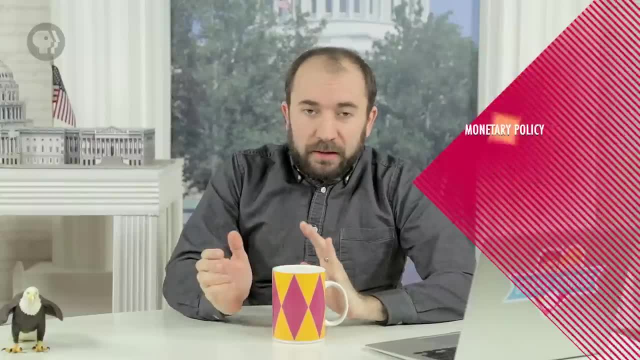 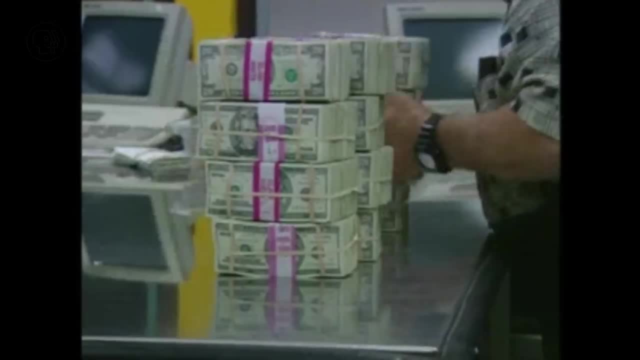 Let's start with monetary policy, because it's not at all controversial. Well, it kind of is controversial, but it's less contentious than fiscal policy. Monetary policy is basically the way the government regulates the amount of money in circulation in the nation's economy. 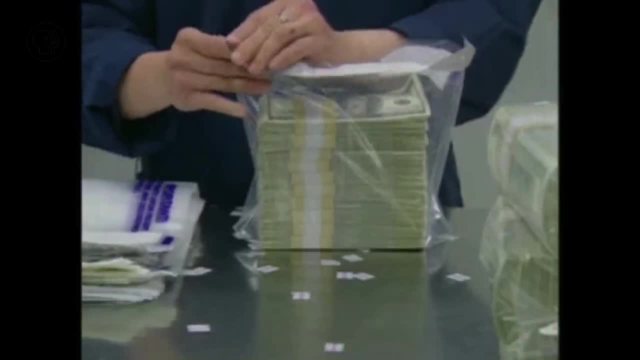 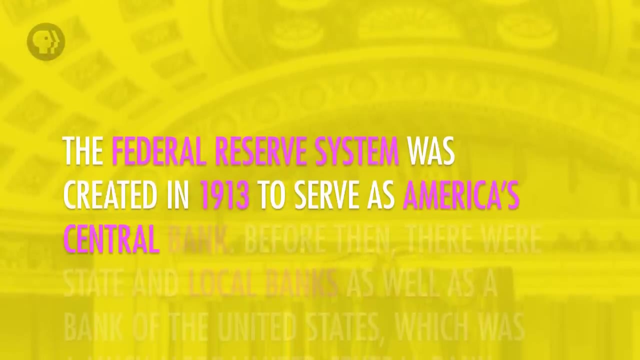 Controlling the money supply is the primary task of the Federal Reserve System, and since it's a little bit complicated, I'm going to talk about the other things that the Fed does first. The Federal Reserve System was created in 1913 to serve as America's central bank. Before then, there were state and local banks as 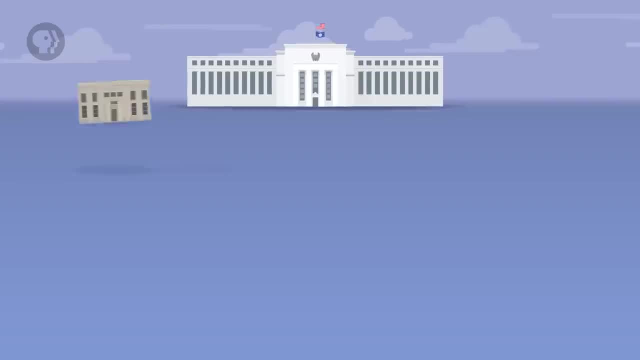 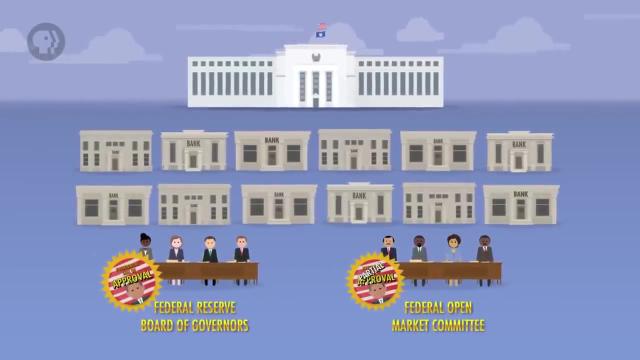 well as a bank of the United States, which was a much more limited central bank. The Fed is made up of 12 regional banks and two boards: the Federal Reserve Board of Governors, who are appointed by the President, and the Federal Open Market Committee, which is partially. 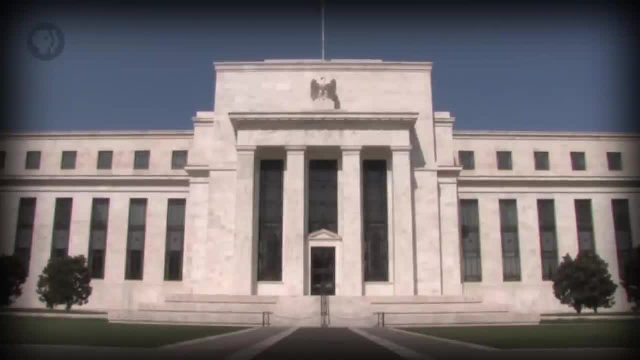 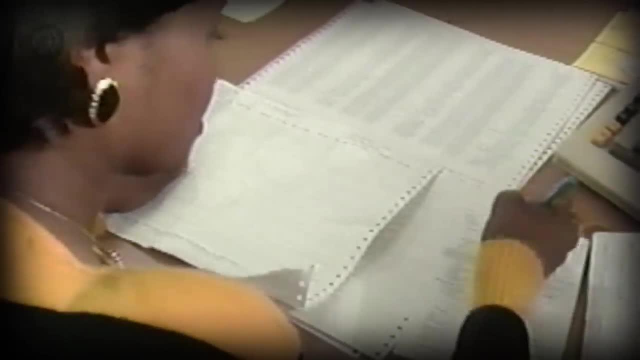 appointed by the President, The Fed has two primary tasks- to control inflation and to encourage full employment- And it has four basic functions, but one of them is way more important than the others. The Fed is responsible ultimately for clearing checks and for the thing the Fed does is loan money to other banks and set interest rates. That's why, when you hear about the Federal Reserve, nine times out of ten it's about interest rates, because that's the main way the Fed controls the money supply. The Fed loans money to banks Sweet. 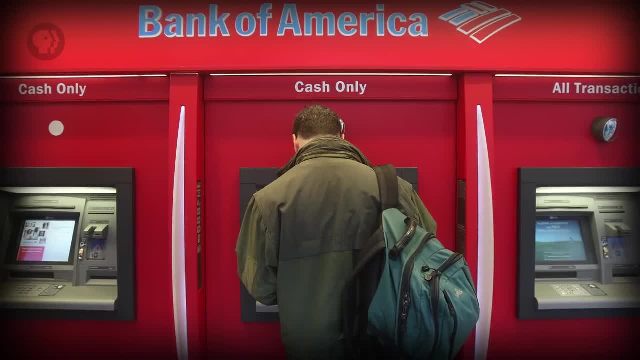 sweet money Which they in turn loan out to businesses and individuals and, like all loans, the Fed charges interest. The Fed sets up the Federal Reserve System and the Federal Reserve System sets the rate on the interest, called the discount rate, and this determines.